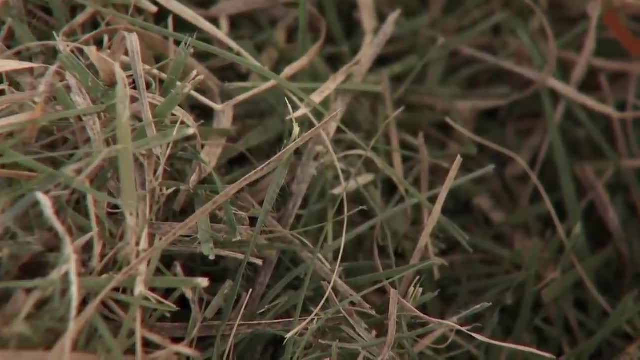 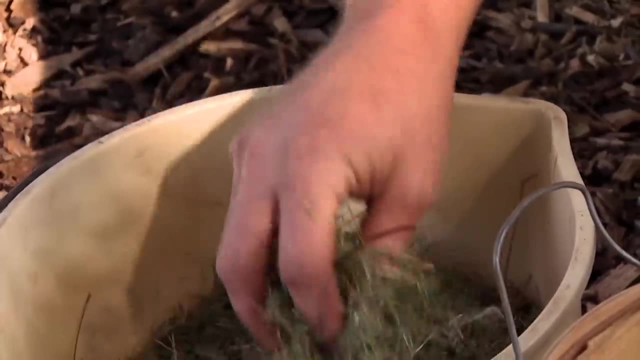 Okay, And one of the lowest is fresh grass clippings. Fresh grass clippings are fairly good. I mean they've got you know cause they're nice and fresh and green And so they're going to have a pretty good nutrient content. The: 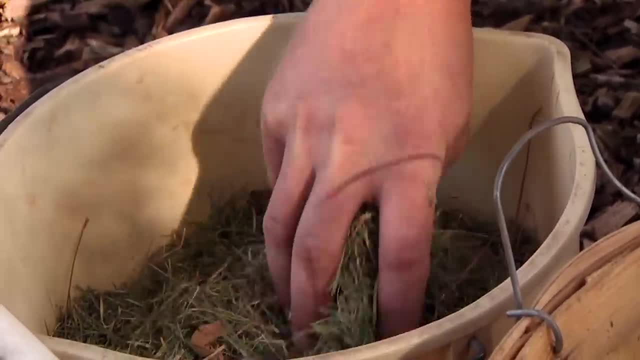 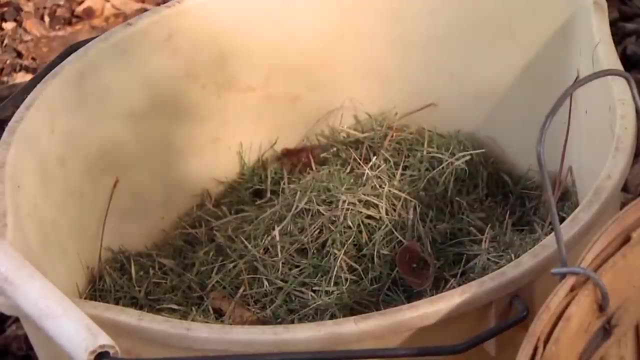 seeding ratio of them is about 20 to one. So you'll apply the these and it'll take longer to release the nitrogen than it would from compost. but it will release and you can build some nutrients from that. but at least you're not bringing. 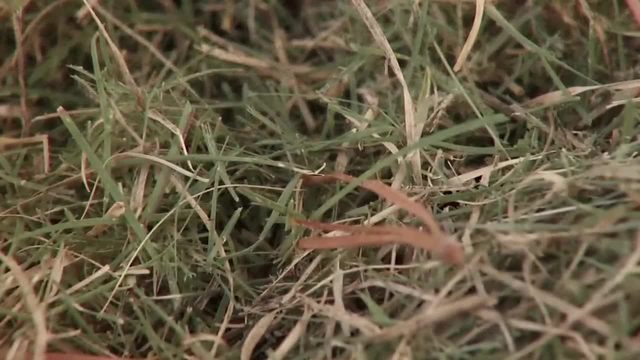 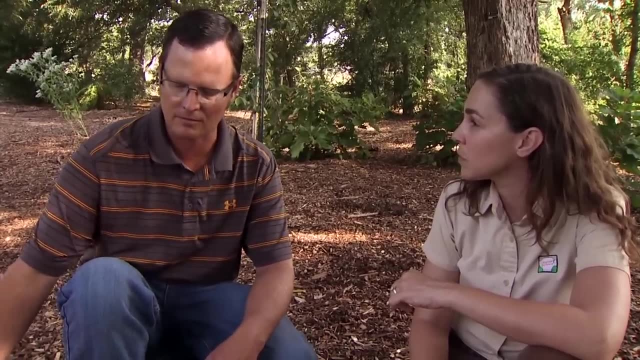 them in from offsite compost. unless you're composting your own leaf, clippings and yard waste, You're bringing that in from offsite, whereas this is just being cycled through your yard, And then the same thing with straw: it's an offsite deal. 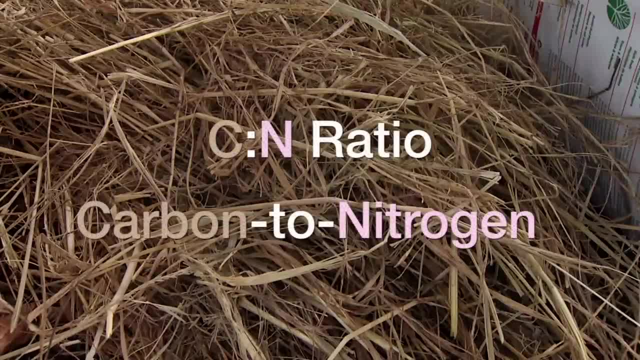 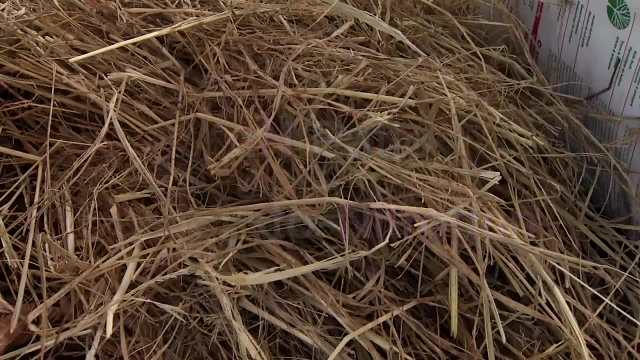 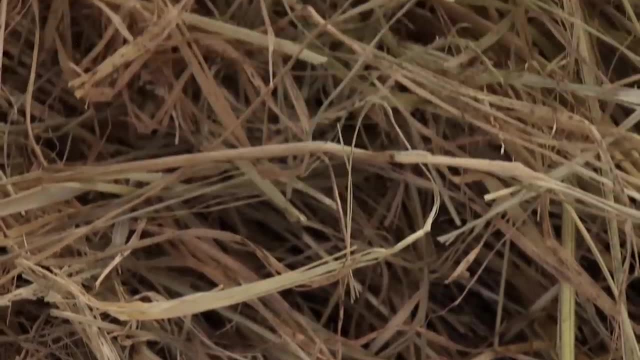 Now you use the term C to N ratio, which is carbon to nitrogen. So we're looking at the ratio of carbon and nitrogen that comes out of the material we're adding. Just wanted to clarify that for viewers, Cause see the microbes, this, this straw or grass, this hay material, it's got a fairly 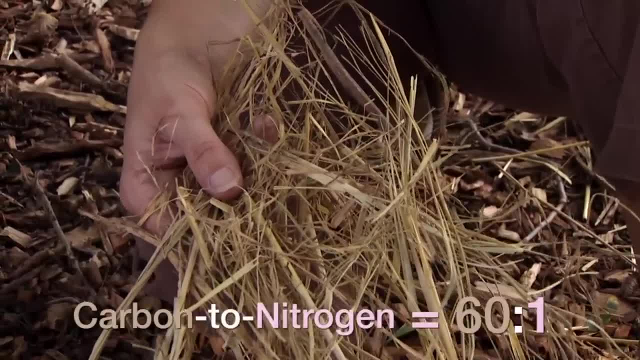 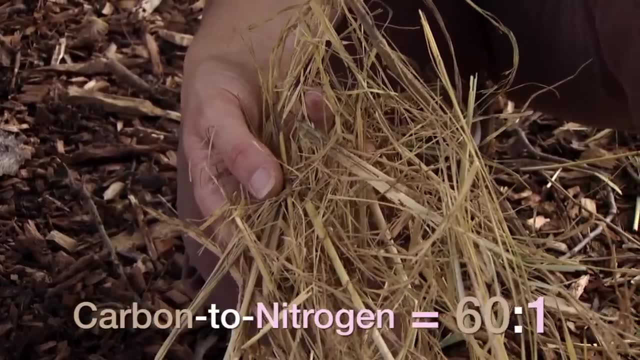 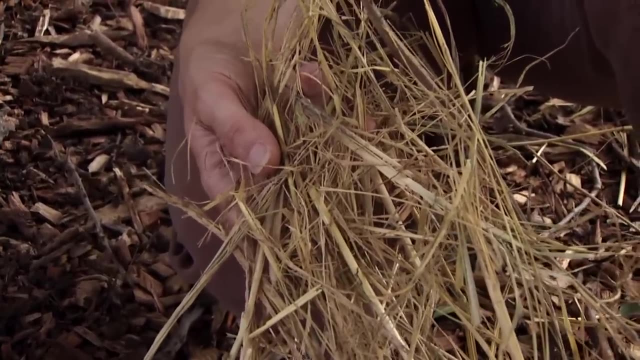 high seeding ratio, probably about 50 to 60 to one or 50 or 60 to one. So that means that it has, say, 60 carbon molecules for every molecule of nitrogen, And when microbes decompose that, they're going to scavenge the nitrogen from your soil and rob it from. 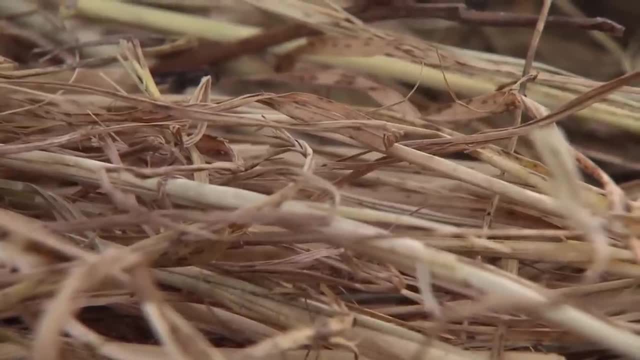 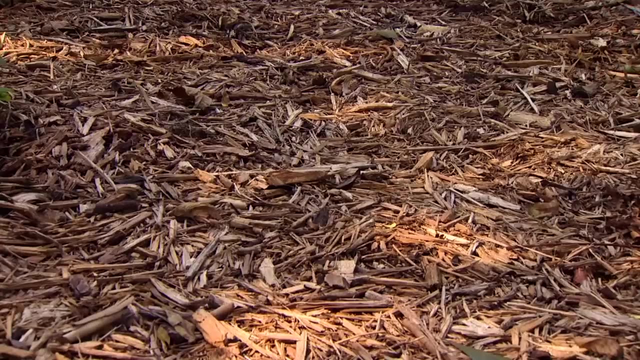 your plants that you're actually trying to grow. So they won't grow and or they'll be yellowed. So we need to be thoughtful when we use a material like that. So before we talk about the nitrogen, which is going to be very important, there's one. 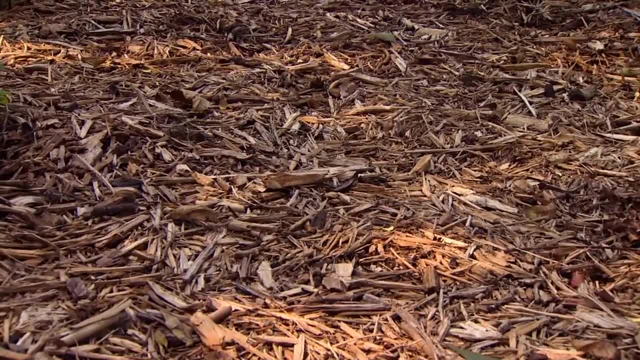 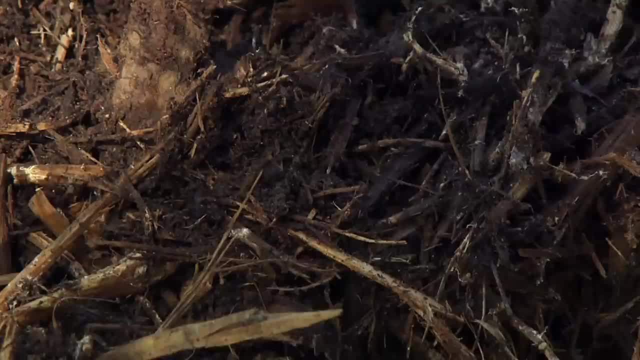 more material, actually two. we're sitting on top of wood chips. Certainly another material we can use. Yeah, And wood chips. you know that's a great mulch. It's a fairly stable organic material because it's hard for the microbes. 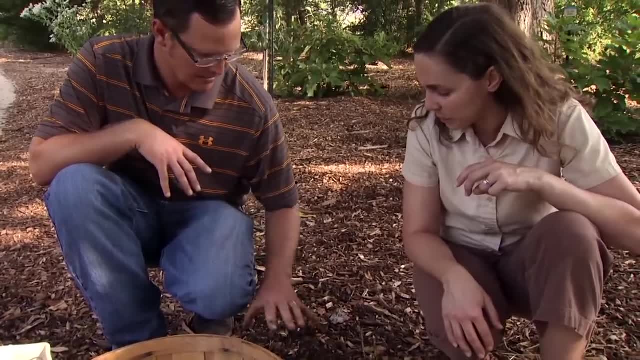 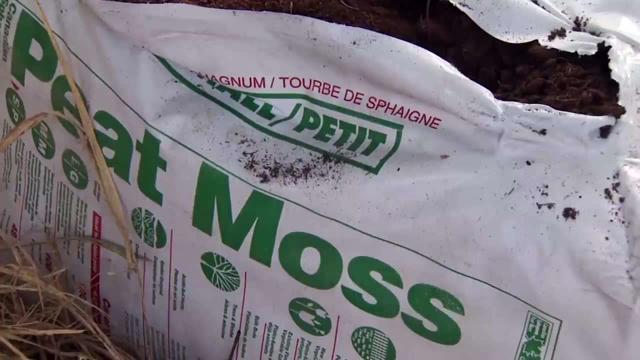 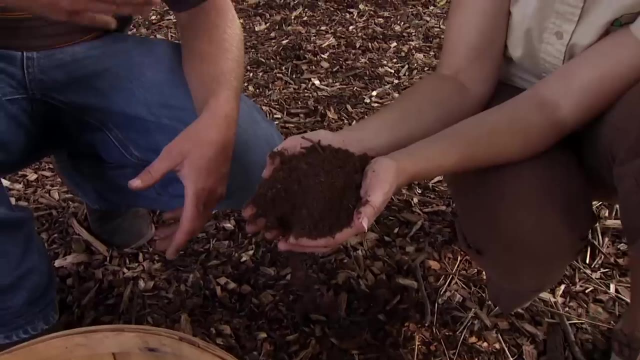 And soil biology to break down, but it will slowly. if you keep it covered with wood chips, that material is adding to the organic condition of the soil as well. The peat moss- and I like peat moss because it's a fairly stable organic matter, meaning that it won't decompose as 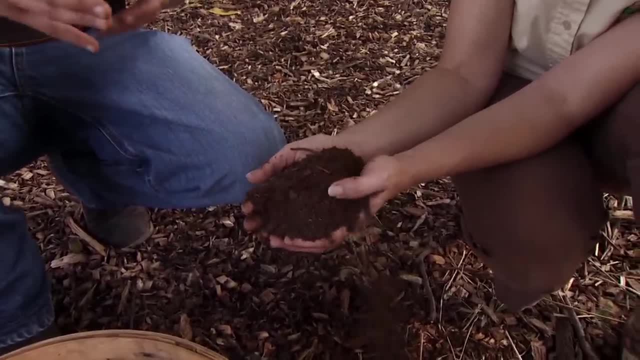 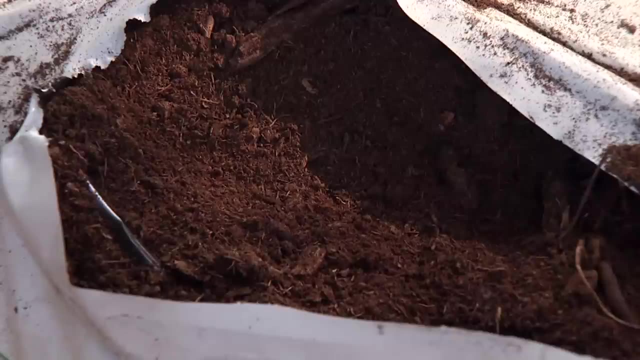 quickly, And so that's the challenge. Organic matter decomposes over time And we want that because that's going to release nutrients and feed the microbial population, but we want it to To be maintained to some extent, And this is a material that's as stable or nearly as 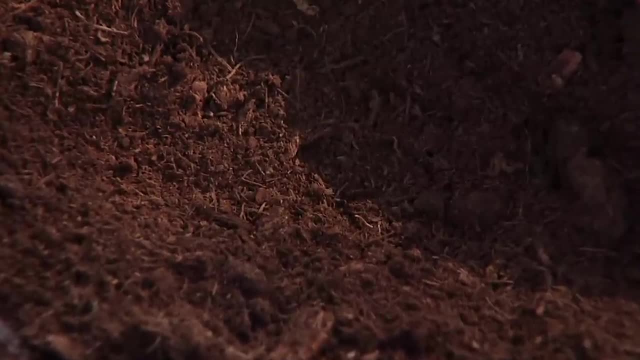 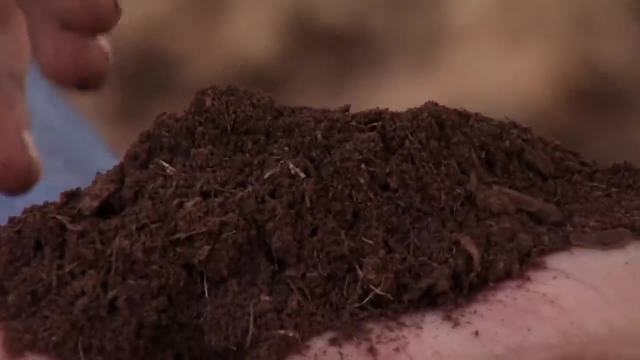 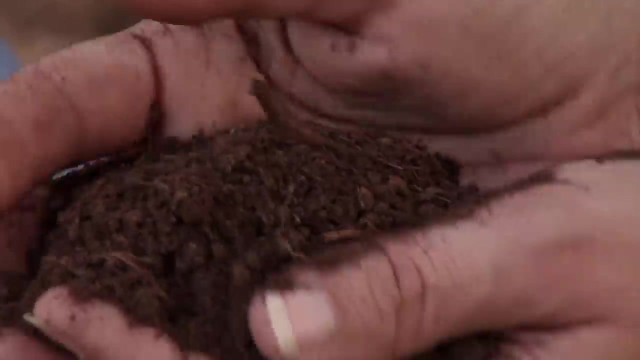 stable as the compost with respect to pounds of organic matter applied. that will persist over time, but it doesn't have as high a nutrient content, So you can apply that without adding a whole large amount of nutrients with it. Okay, So we won't get that: phosphorus build up and potassium build up. 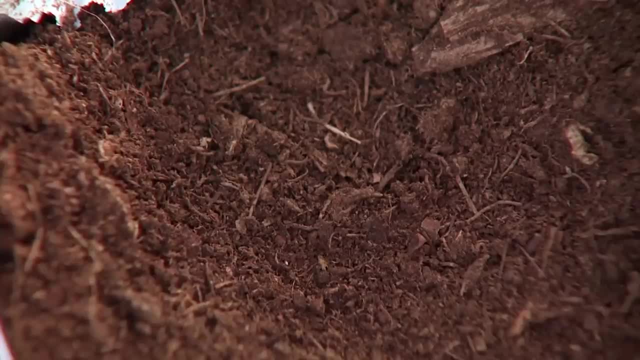 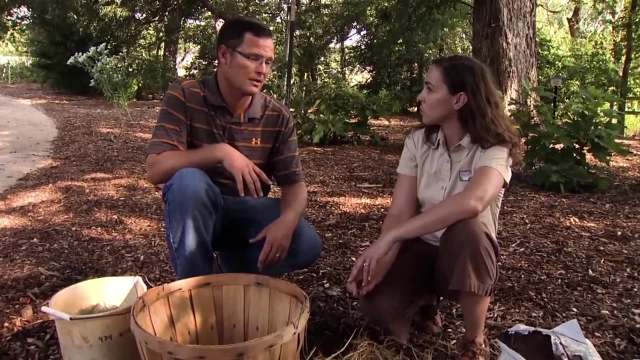 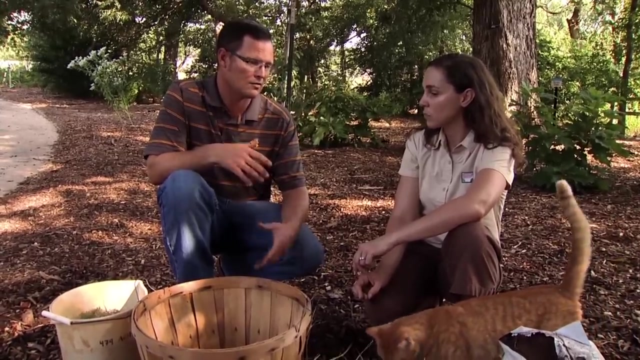 But yet it's a fairly stable organic matter material that will build water holding capacity, Yeah, And improve the drainage of clays and things like that. But you have to be thoughtful too, because it will drive your pH down, particularly in a sand If you've got a heavy clay soil. 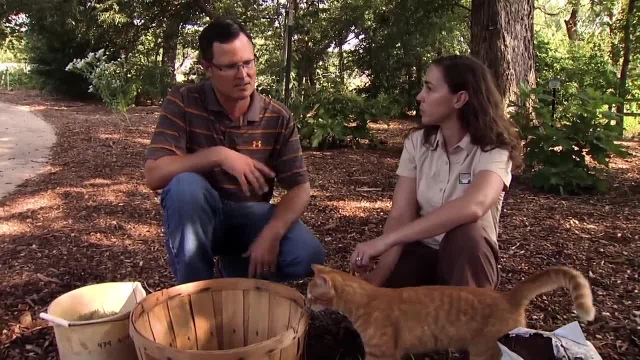 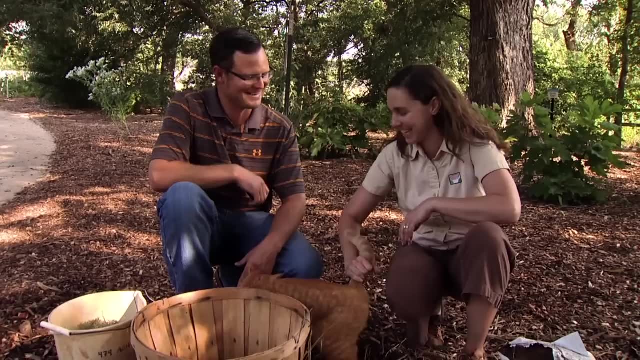 not so much because it's more buffered, But these are the options. They have pros and cons that can be used. Our garden cats decided to join us for this segment. Oh yeah, All right, cowboy, That's good. So one thing we want to put. 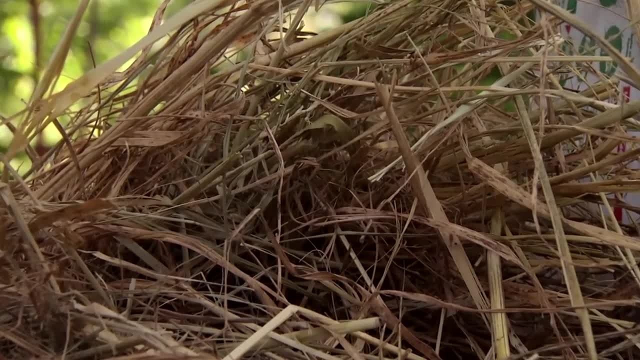 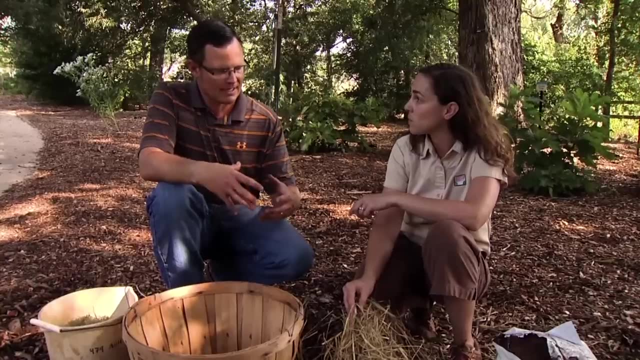 These raw materials are really good to be putting down in the fall. Yeah, They'll decompose right into our soils, Exactly, And they take time to decompose and break down and do what you want, But during that fallow period they'll keep the soil open, right. 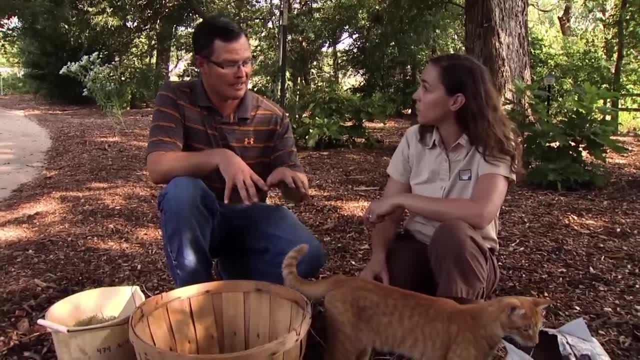 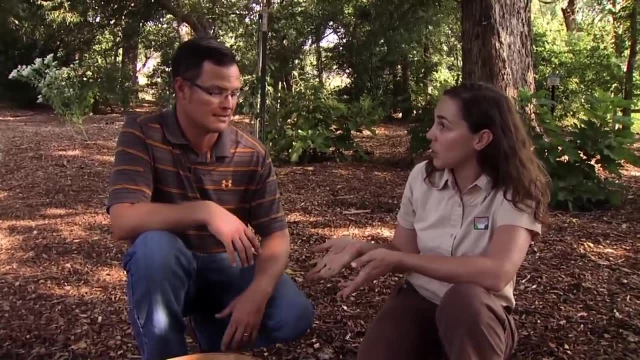 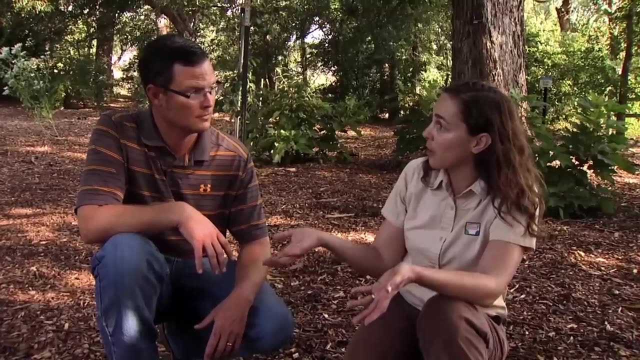 Mm-hmm. But the challenge is how that raw material is going to affect your nutrients that you're going to want to go into your garden plants. Right, You can see that sometimes A garden that's- Yeah, It's been mulched, say, with grass clippings or leaves, and the plants are struggling because 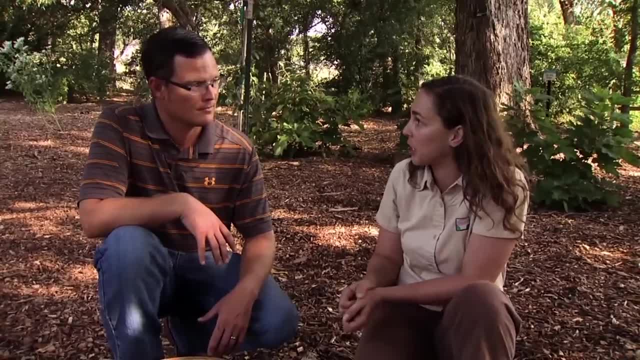 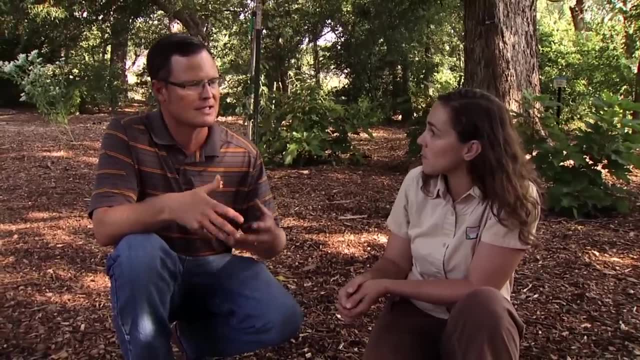 they don't have enough nitrogen because the nitrogen is being used to decompose. that, Yeah, And so you could put those in just prior to your off season and let them decompose, and that'll kind of stabilize the nutrient condition, versus putting them in in the spring. 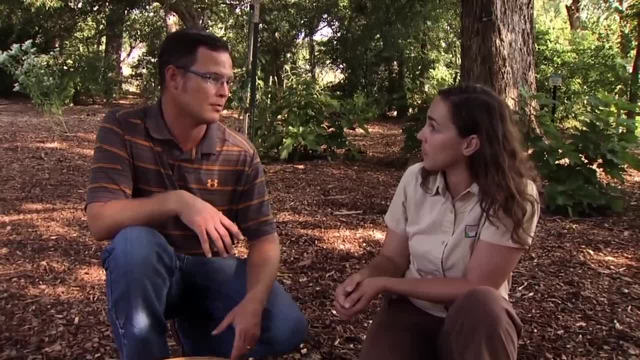 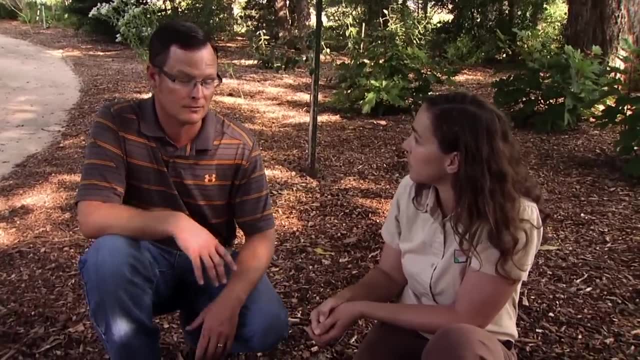 and then they'll be decomposing while your plants are trying to grow, and that's kind of a problem, like you say, And so you'd want to use something like a composter. Yeah, And that's going to be used in the spring because that's going to have readily available.